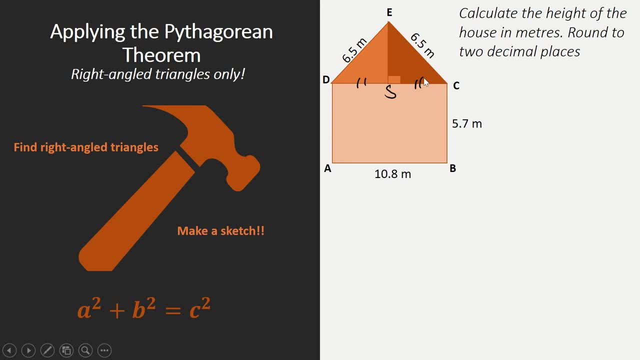 can see as well, is that this is equally long to that side. So that means that I'm going to divide ten point eight meters by two, which gives us five point four meters and five point four meters meters. Now we have enough information to calculate the height of the roof, since 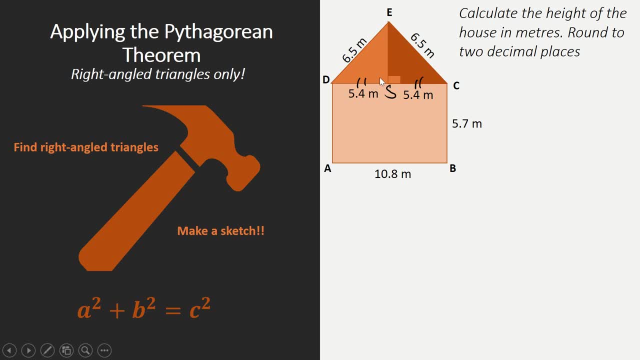 we know that we have a right angle triangle, so we can use a Pythagorean theorem and we know two out of the three edges. So our first step is just to write down our Pythagorean theorem. So a squared plus b squared equals c squared. 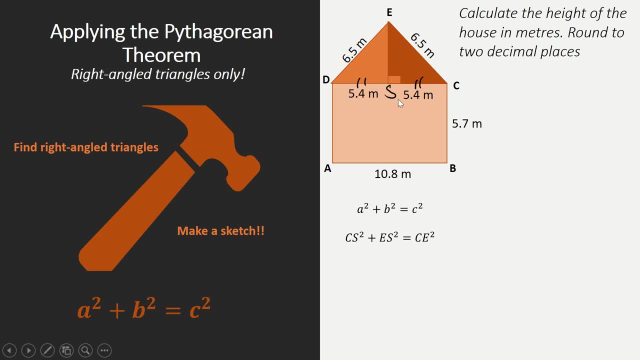 So c s squared in my case, because I choose the letter s, you can choose whatever you want- plus e s squared is c e squared. That's because we know our longest edge, so the hypotenuse is opposite to our right angle. If you write: 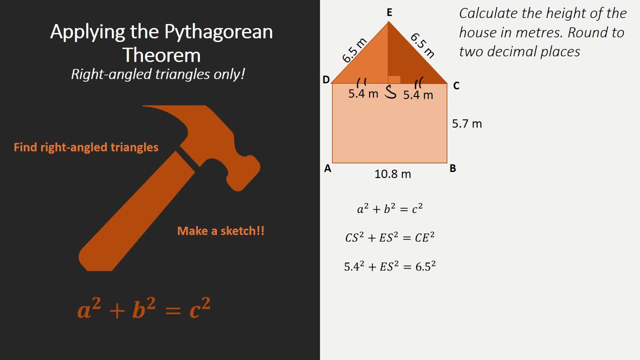 down everything with the letters. you're going to fill everything in. So 5.4 squared plus e s squared equals 6.5 squared. So that's it. Thank you for watching 5.4 squared. so 5.4 times 5.4 makes 29.6, and 6.5 times 6.5 makes 42.25. 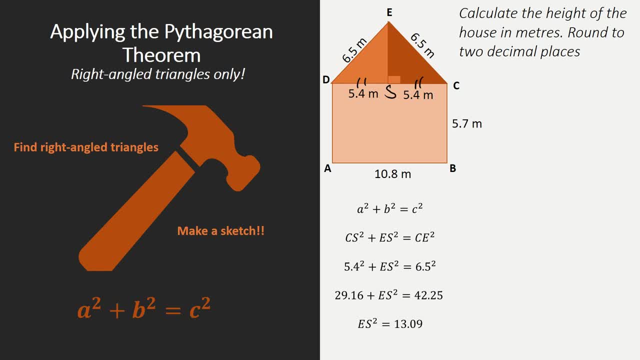 use the balance method, so that means that you're going to subtract the 29.16 on both sides to get es squared equals 13.09. we want to know what es is and therefore we take the square root of 13.09, which is 3.618. 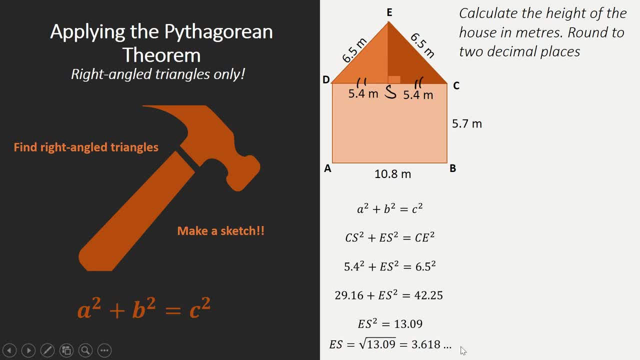 dot, dot, dot, dot dot. it has more decimal numbers. please never, ever round when you're not done yet. so this is not our final answer, so we are not allowed to round. so so we're just going to calculate with this whole number and instead of just writing down the 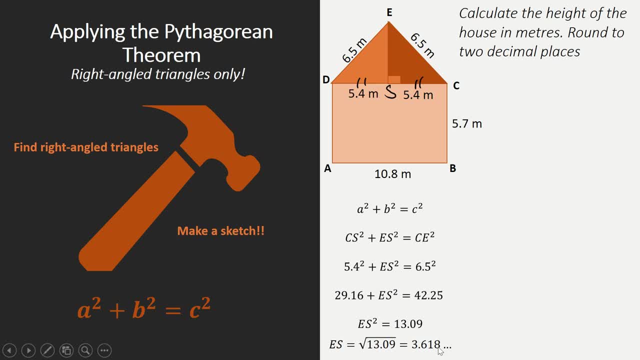 decimals or all decimals. i write down three or two decimals and then i use three dots. all right, so the height of our house is a bc plus es, because we want to know the height from the ground to the top. so it's 3.618, and then all those decimals plus 5.7.